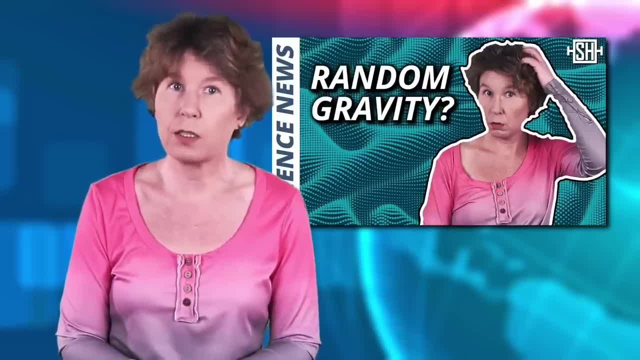 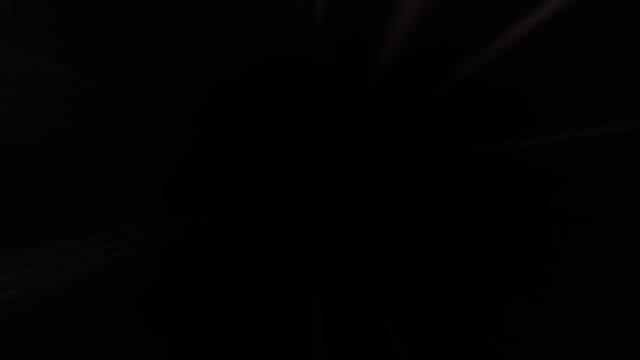 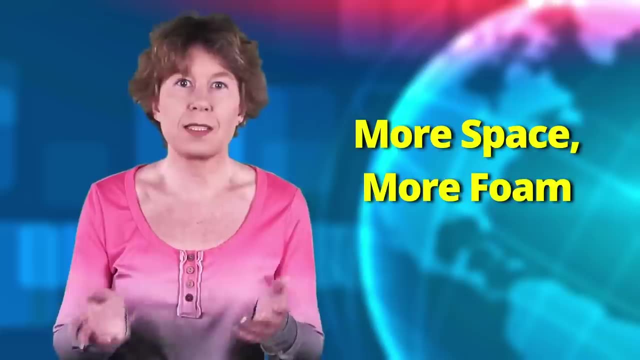 fluctuations should induce the collapse of the wave function, And that may or may not be correct, But generally you expect that the quantum foam affects particles more the longer the wave is. This is why there have been a bunch of experiments that look for distortions in signals from very 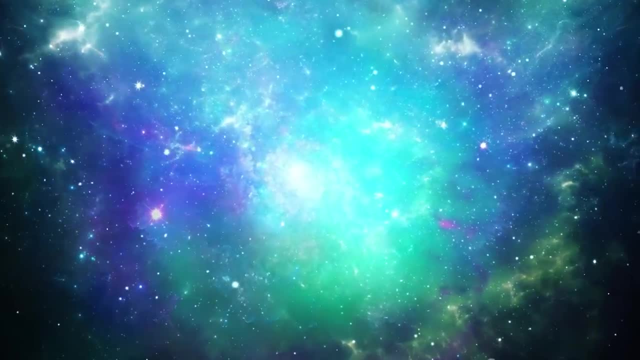 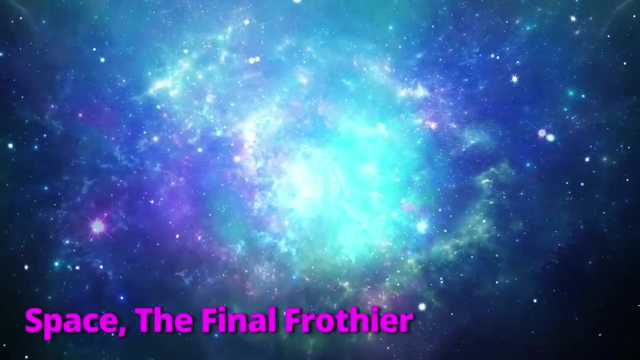 distant sources, And when I say very distant, I'm not talking about your fifth cousin, John. I'm talking about billions of light years Particles that have literally crossed the entire universe. Several experiments looked for it, and you already know that they didn't find. 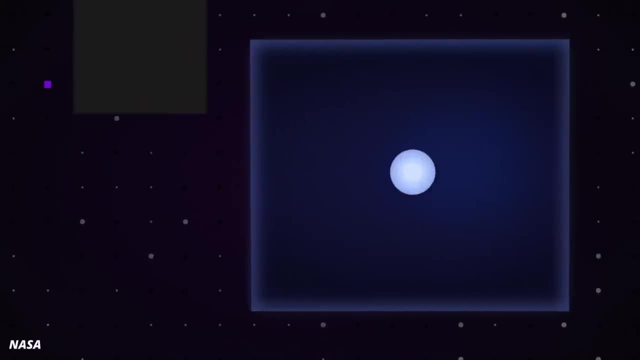 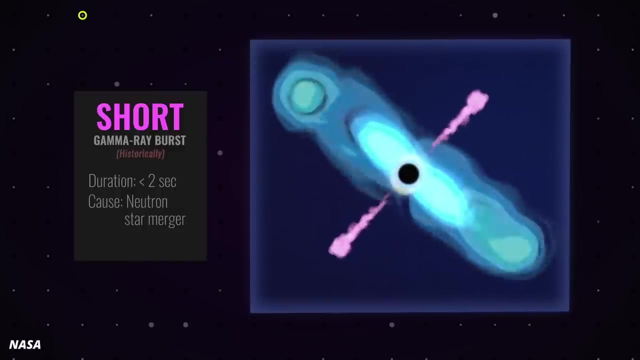 anything, because otherwise you'd have heard of it. For this, one usually looks at emissions from gamma ray bursts and then checks whether light of different frequencies arrives at the same time on earth. This is because light should always move with the same speed, But if it was affected by 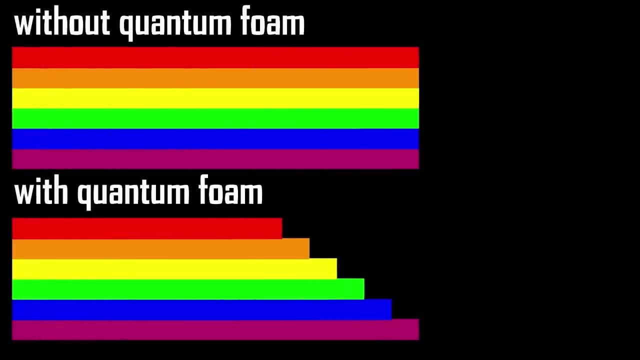 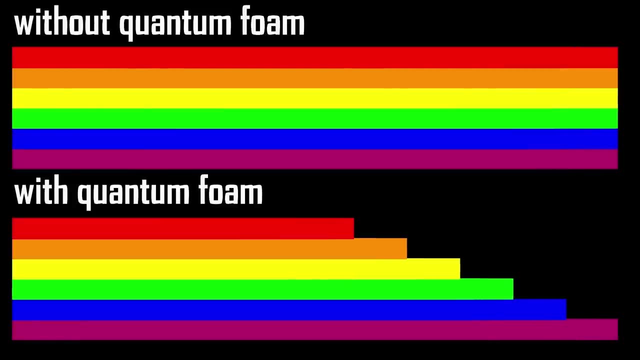 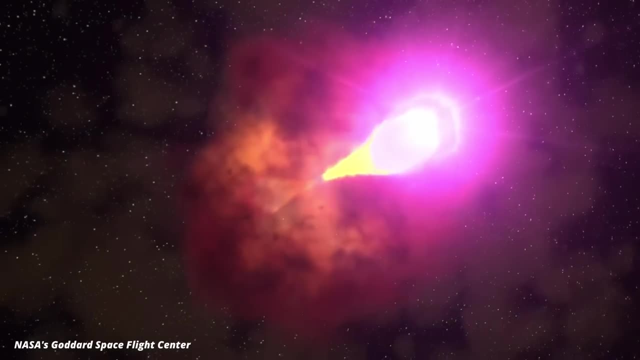 quantum fluctuations, you'd expect it to be more affected the higher the energy, because that means it has a smaller wavelength, which makes it more susceptible to the foamy stuff. The issue with looking at gamma ray bursts is that you don't know exactly when the light was emitted in the first. 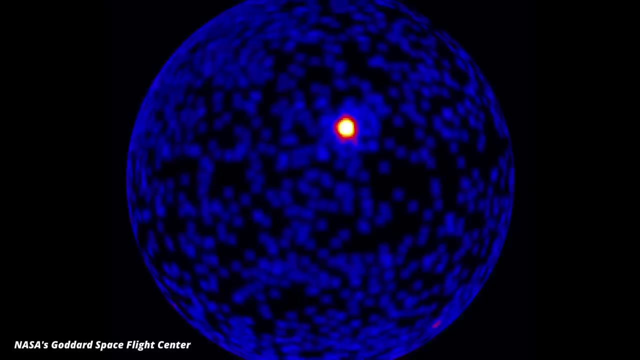 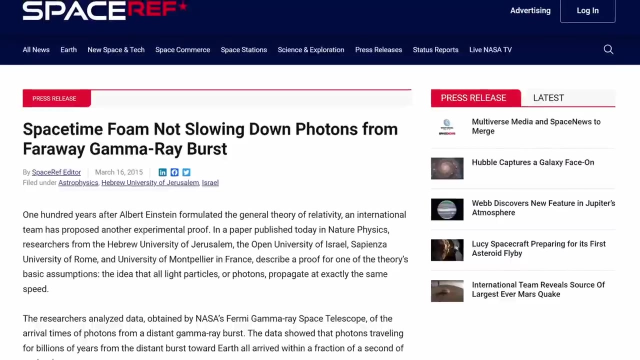 time. Maybe it didn't all start travelling at the same time. So while that works in principle and people have done it to say, well, the fluctuations can't be larger than so, and so the results have not been all that super interesting. 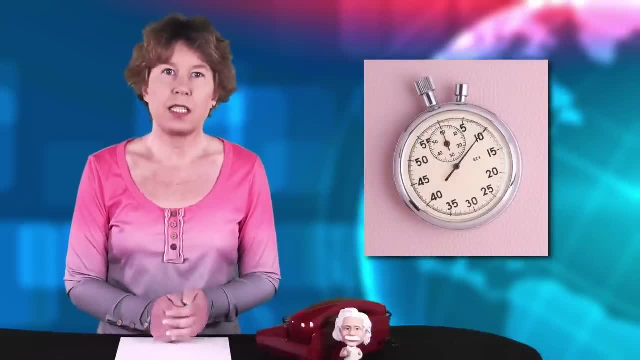 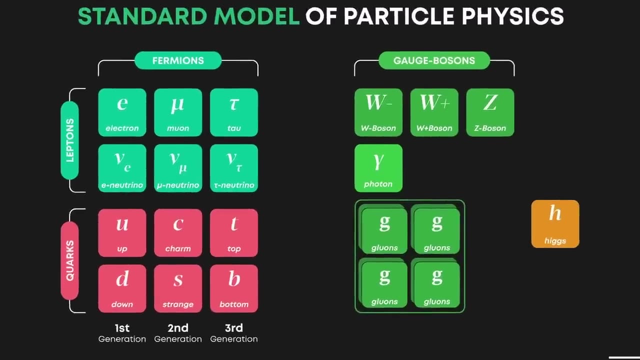 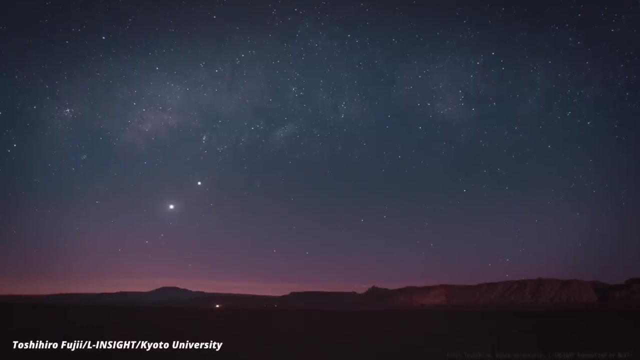 Enter the new experiment. It's a very clever idea which removes the problem that you don't know when different particles started travelling, by using a particle that changes as it travels, The neutrino. The neutrinos they're interested in are from cosmic rays, usually protons that hit atoms in the upper atmosphere, But the neutrinos that 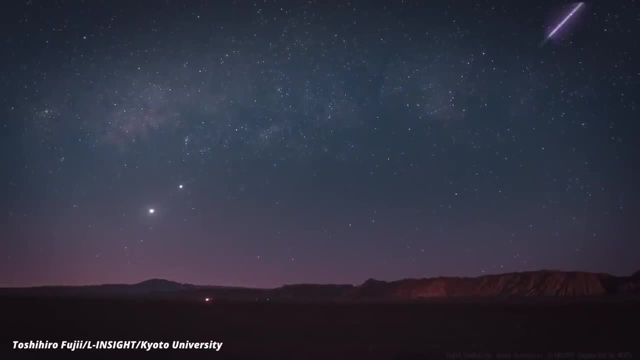 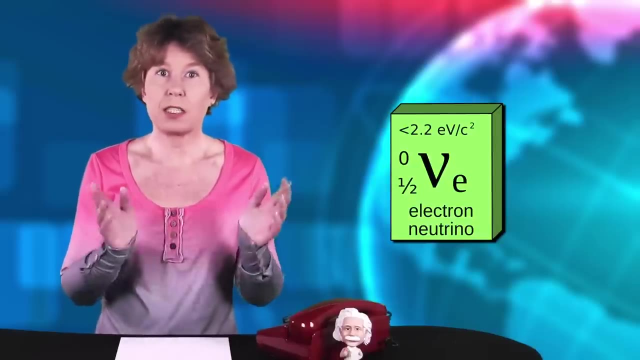 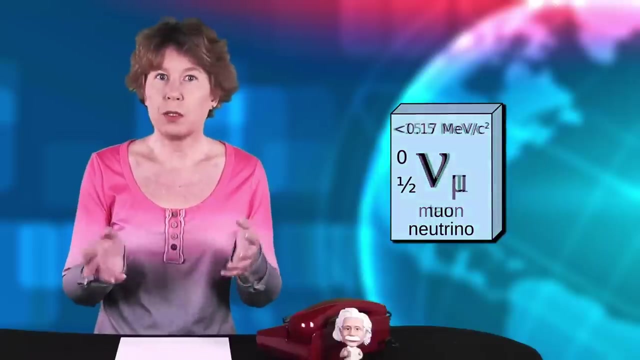 are created up there don't stay that way. They oscillate into another type of neutrino. What this means is that if you start with one type of neutrino, say an electron neutrino, then after some time you have a chance of finding a muon neutrino instead. Wait some more and it 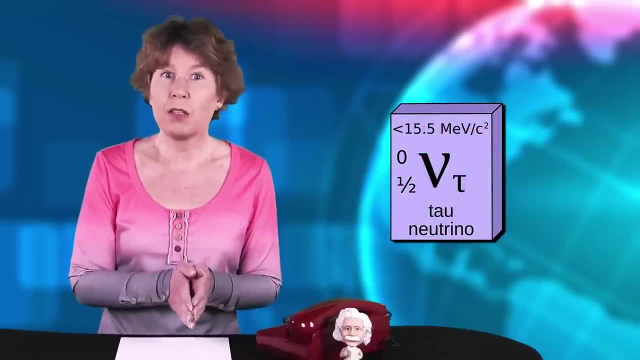 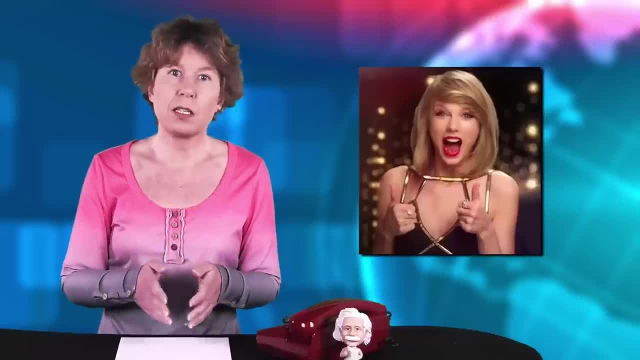 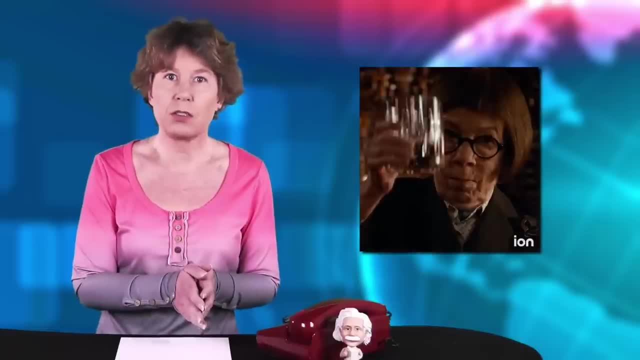 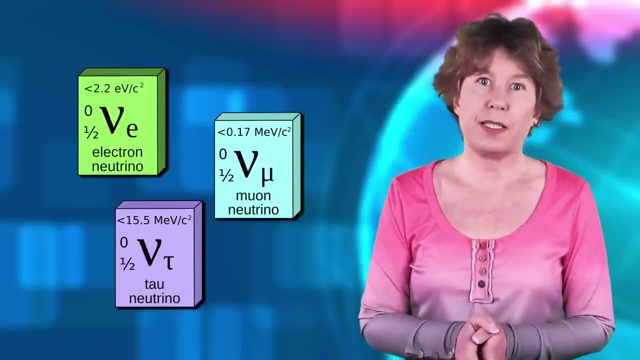 So the tau neutrino turns back into an electron neutrino and by the time you're back home, you have your wife back. The thing is now that these oscillations are pure quantum effects, which means they're very fragile and get destroyed easily, For example. 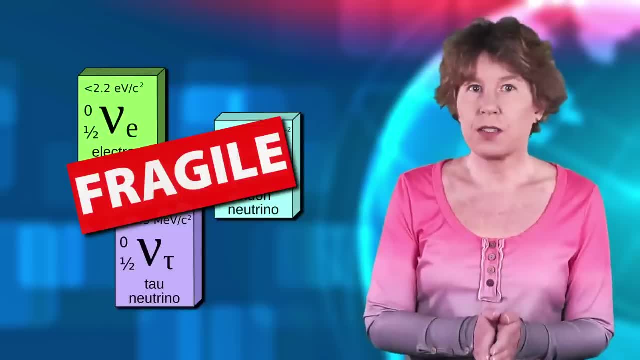 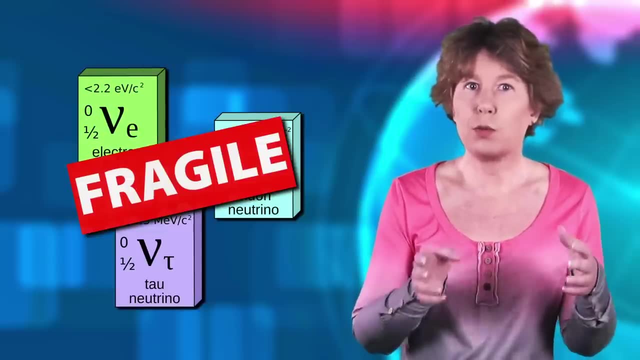 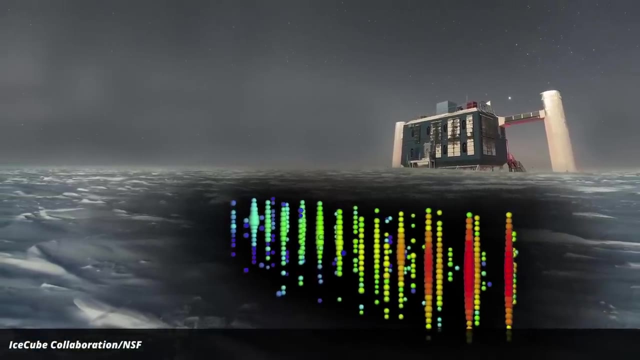 by fluctuations in space, And so if neutrinos encounter the space-time foam on their way down to Earth, that'll change how many neutrinos of which type you detect down here. For this new measurement, they're using the IceCube Neutrino Observatory at the South Pole. 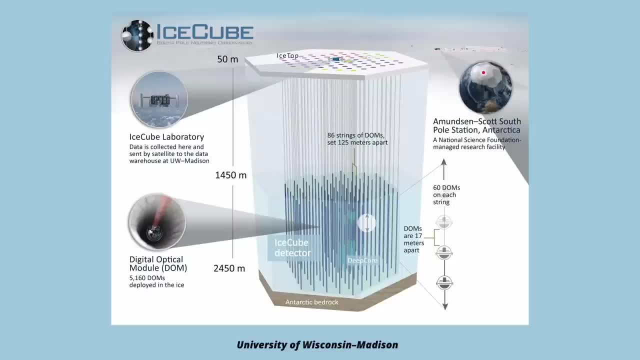 They have about 5000 detectors that are sunk down into 86 boreholes in the ice more than a kilometer deep. It's amazingly cool, in both interpretations of the word, because there's very little noise down there. The IceCube detectors are looking for events that come. 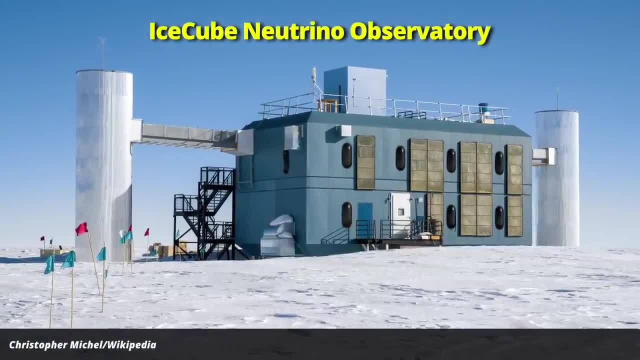 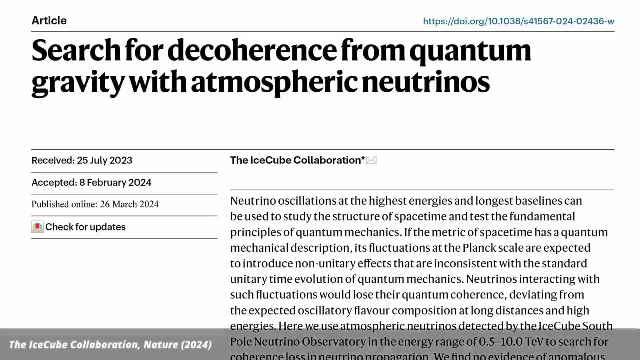 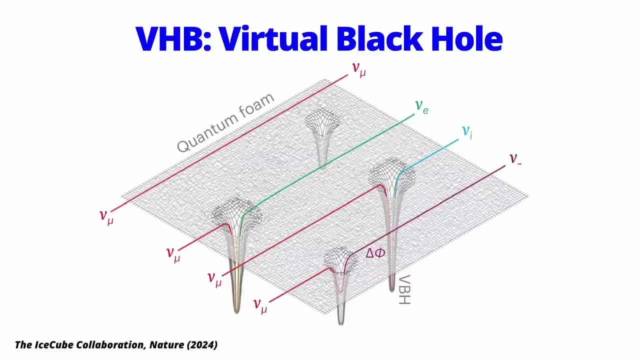 up out of the Earth from the north because there are few particles which can go through the entire Earth undisturbed, like neutrinos. In their recent paper they report that they looked for evidence of this decoherence from the space-time foam in data from about. 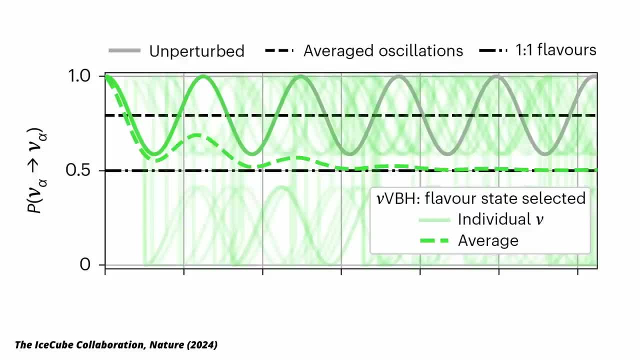 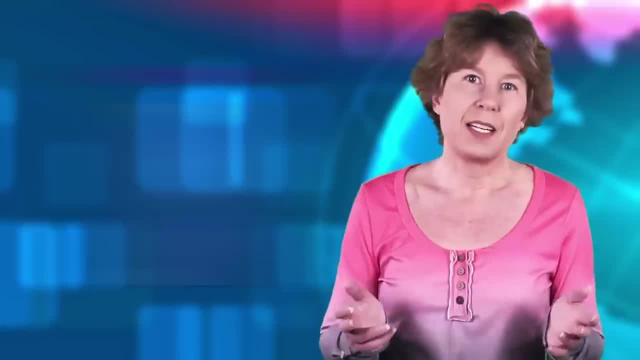 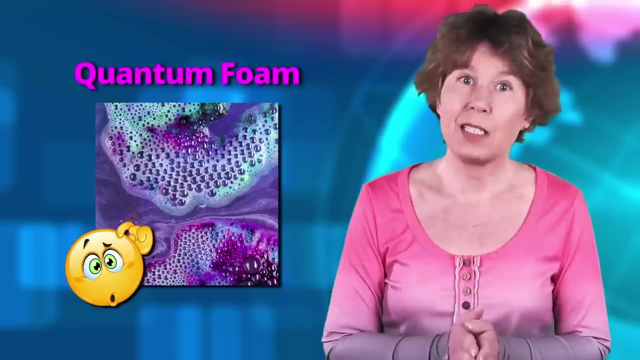 300,000 neutrinos and didn't find it. However, they really just did this to calibrate their detector and will now be launching their real search. I have to admit that I've always been somewhat skeptical of this quantum foam stuff, for it doesn't sit easily with. 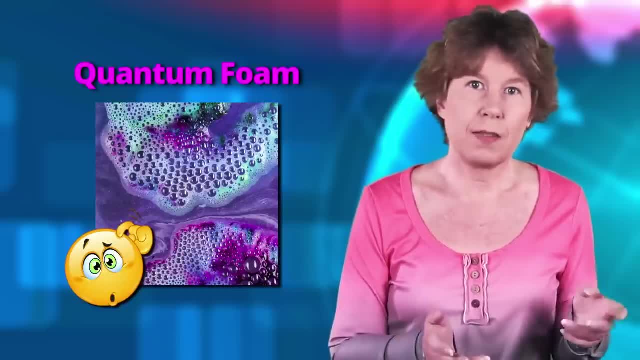 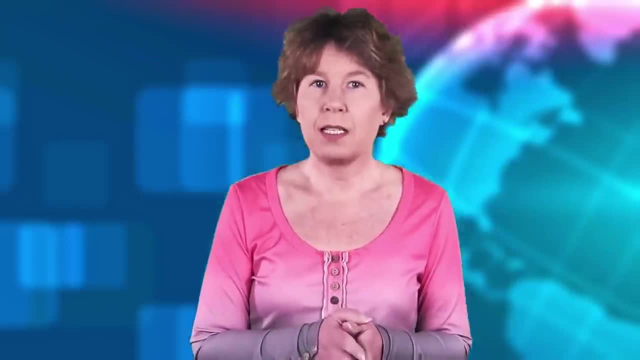 Einstein's general relativity. but then again you could say that not sitting easily with Einstein's ideas was kind of the point of doing it Well, in any case, personally I'm more excited about the tabletop experiments that'll be looking for quantum gravity, hopefully within the next 10 years. 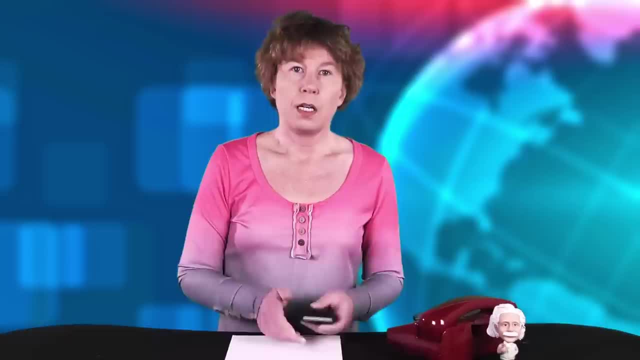 or so, but this one is clearly one to watch out for. I recently opened a physics textbook and found a 200-year-old study on quantum gravity and I found that it was a very interesting study. and I found that it was very interesting and I found that it was a very interesting study. 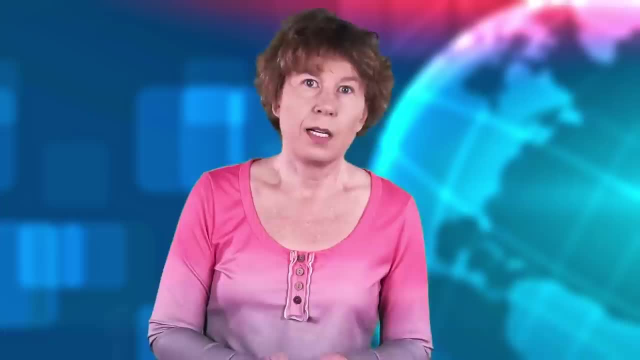 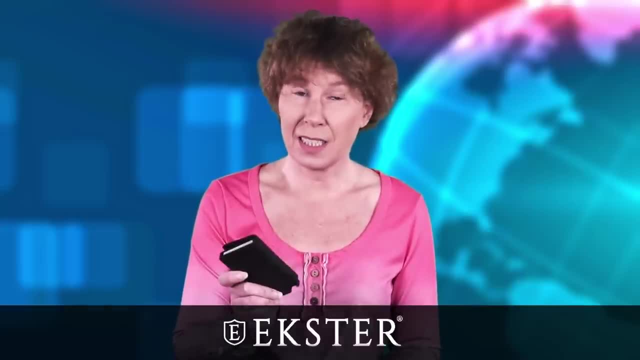 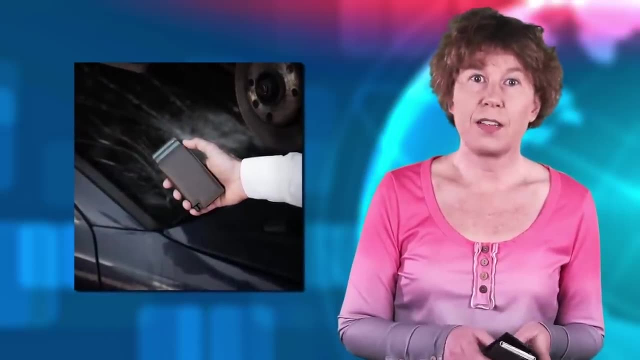 and let me show you what I've found, because I think you'll like it. This extra wallet is the perfect fit for my purposes. You see, the major reason I didn't have a wallet is that they're huge and bulky, But this one is about.